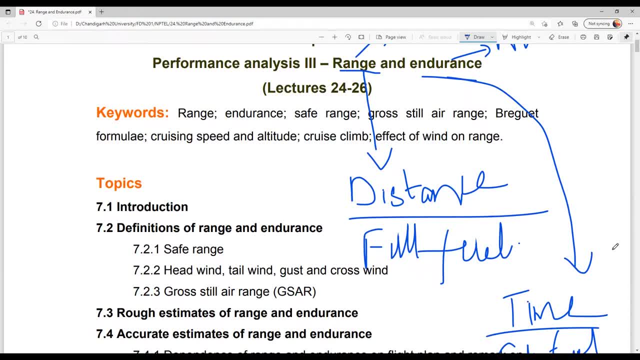 So if you are not worrying about the distance, but if you are thinking like how much hovers or how much Like time Right, So I can travel with my car with full fuel, So that is called as endurance, Endurance of your car. 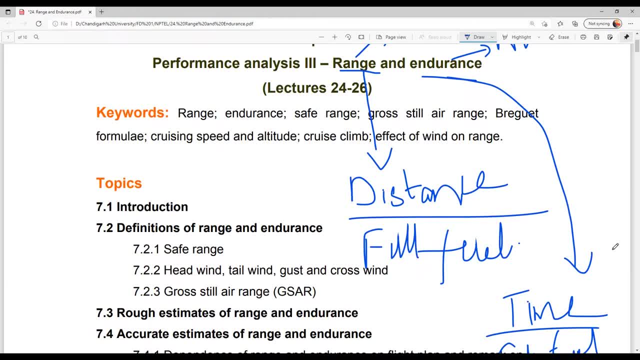 So similarly, that is for your aircraft. Okay, Right, So here we are going to see some additional factors about range and endurance And also we will be solving a problem. So, as a general people, what I will expect For full fuel, For full fuel? 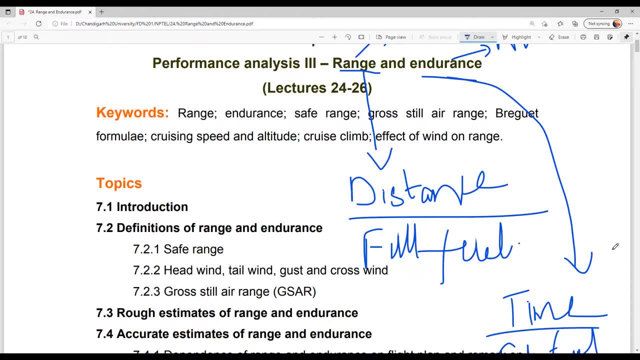 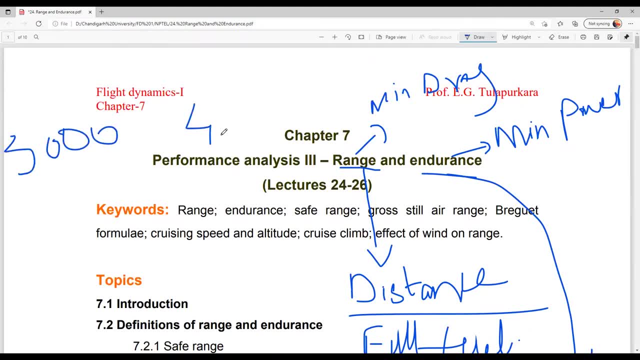 I will expect more distance, Right? So suppose there are two aircrafts, So one aircraft is giving only 3000 kilometers And another aircraft is giving 4000 kilometers Range, Right? So what I will prefer, I will obviously go for 4000 kilometers. 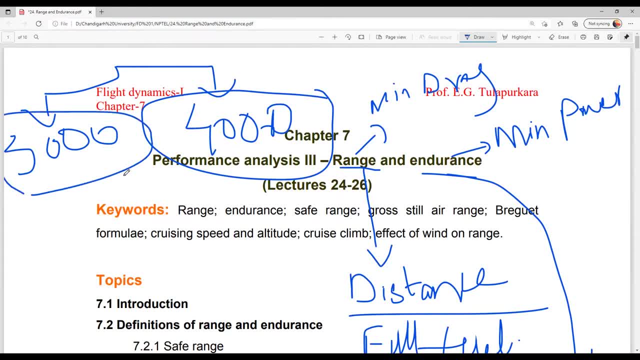 Because it is giving more range than the another aircraft, Right? So range, If I am seeing range as my parameter, Which is required for my aircraft, Then I have to choose with minimum drag condition. I have to design with minimum drag condition. 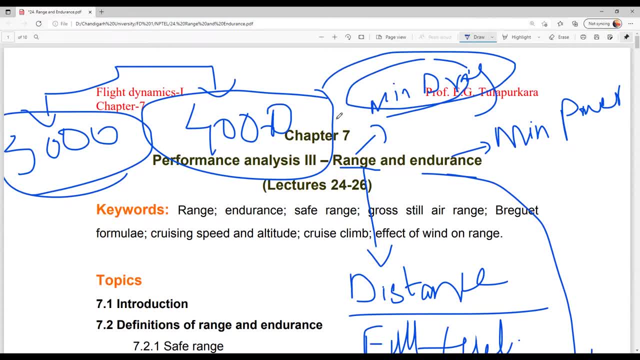 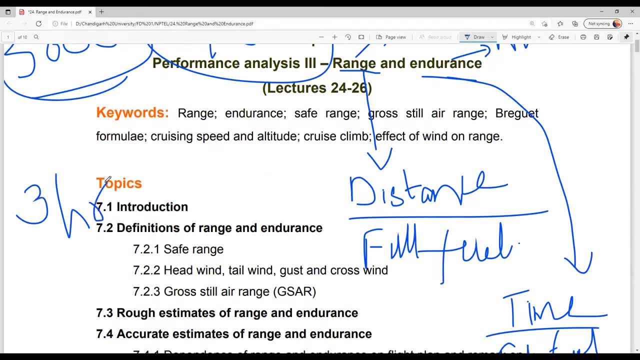 Obviously, the pilot also need to be informed with the parameter. So again, I am going to compare with another aircraft Which is having 3 hours endurance time And another one is having 5 hours endurance time. So what I will prefer? Obviously I will prefer 5 hours. 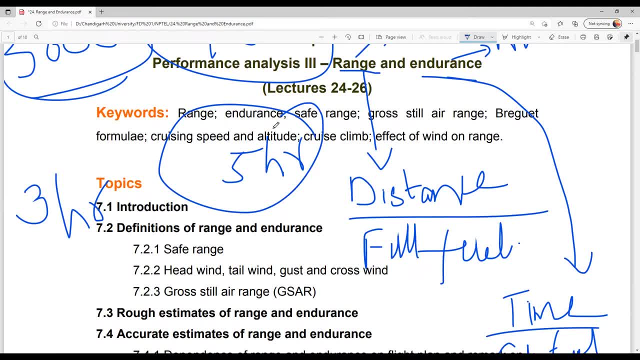 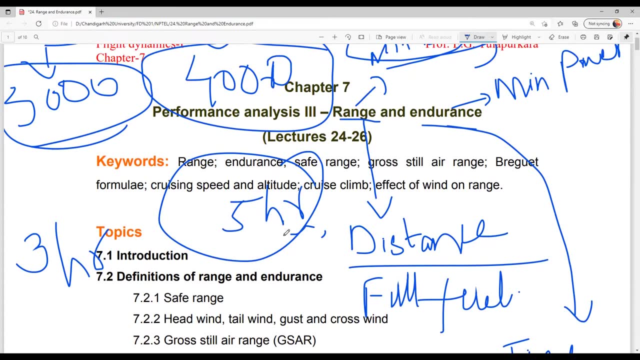 Because I need to Fly for longer time, Right? So that is an advantage for us. Having maximum range and maximum endurance, That is advantage for us. So we have to go for maximum range And maximum endurance. So when we want to have maximum range, 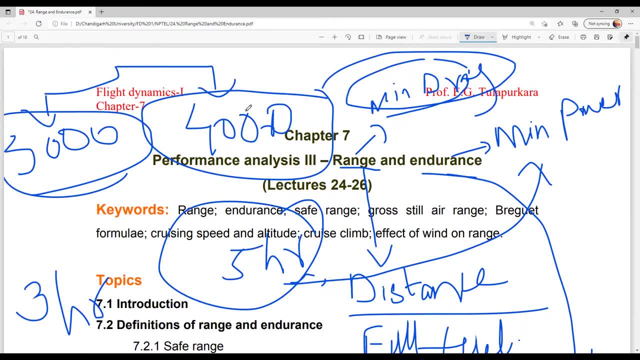 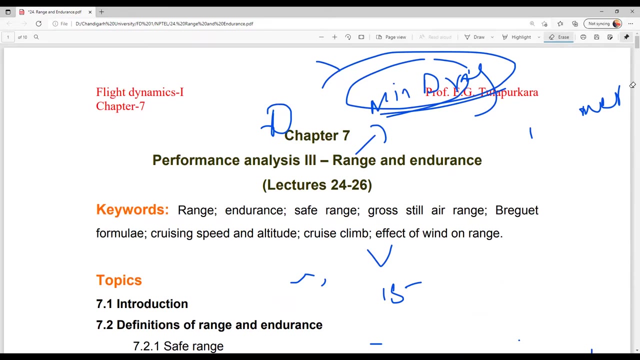 We have to fly with minimum power. When we maximum endurance, When we want to have maximum range, Then we have to fly with minimum drag. Maximum endurance, Minimum power, Maximum range, Minimum drag. Okay, Fine, So let's see how we can calculate the range and endurance. 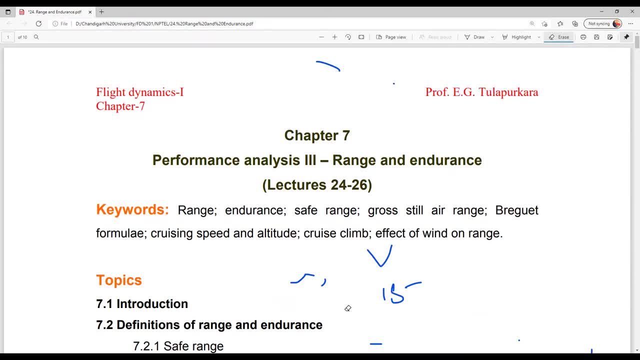 So there is a formula called Brecquet formula, Brecquet formula, So please remember that in your exam also there might be some questions will be there- Brecquet formula. So Brecquet formula is nothing, but it is used to calculate the range and endurance of your aircraft. 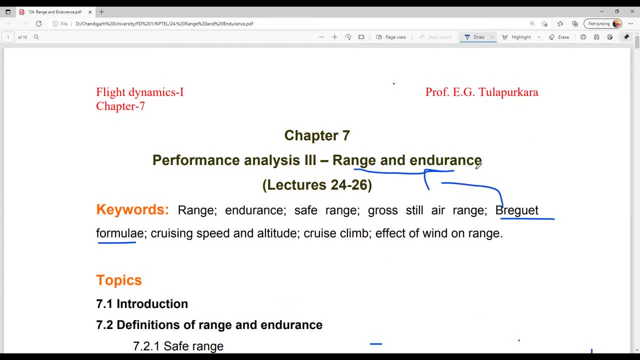 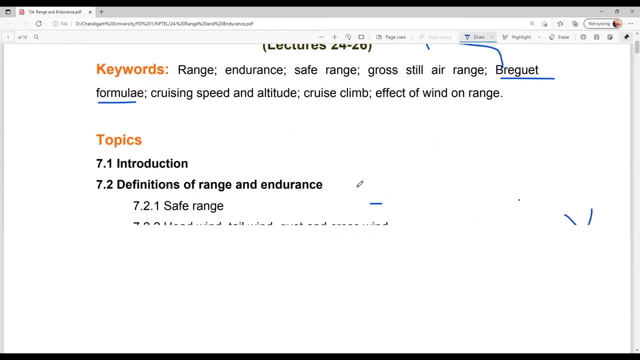 Range and endurance of your aircraft. Using Brecquet formula, you can calculate range and endurance. Using Brecquet formula, you can calculate range and endurance. Range and endurance of your aircraft- Right. So what are the parameters we are going to see? 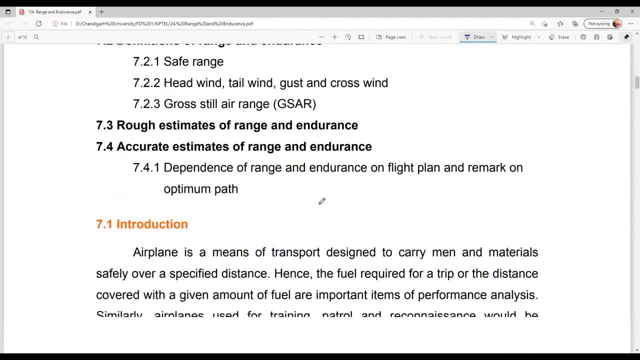 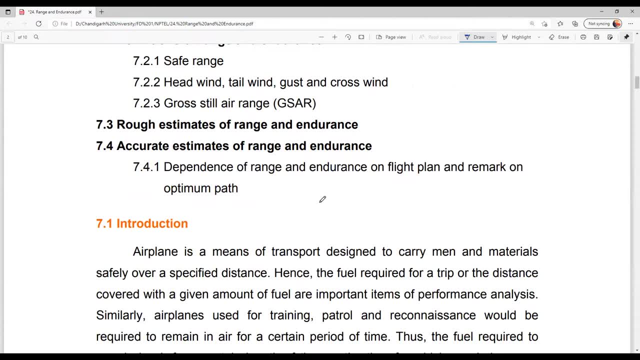 Like additional parameters, Let's say one by one. Till now, That is, in the current scenario, The aircraft's range will be measured with gross, still air range, GSAR. So what is this? GSAR means We have flight path plan. 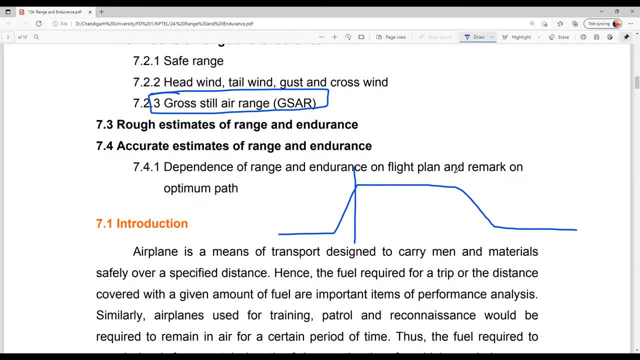 Right. So this is our cruise. So already we have discussed that We are going to fly longer time in our cruise condition Right Cruise. So when the range is calculated with the cruise alone. When the range is calculated with the cruise alone. 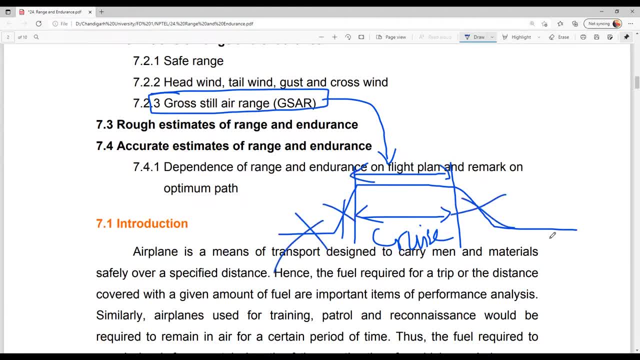 Neglecting this climb. take off, descent and landing. Just, we are going to consider the range from cruise Initial cruise to final cruise point That is called as GSAR, Gross, still air range. Air range means when we are flying in the steady state level cruise. 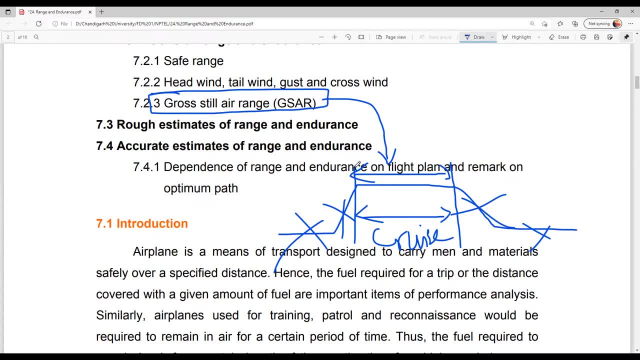 But we cannot always predict the wind direction Right. So wind direction cannot be predicted. So headwind might be there, Tailwind might be there, Sidewind might be there, Crest and crosswind will be there Right. So all this type of wind directions will impact the range and endurance of the aircraft. 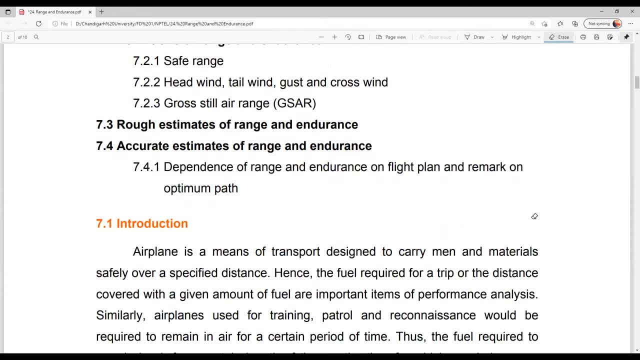 Right, How come it will impact? So let's say you are driving a bike or car. Right, So when you are moving against the wind, Against the wind direction, You cannot move with higher speed. Right, Suppose you are going in a road. 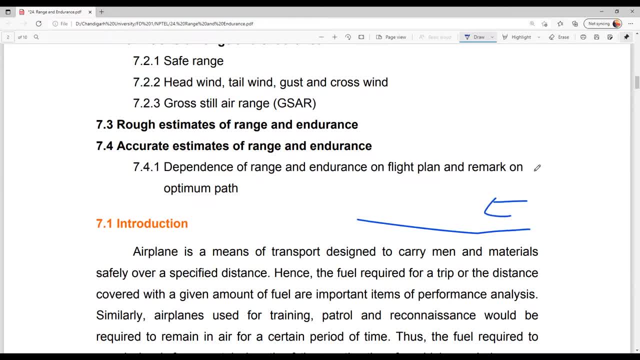 In a car. Okay, And the wind speed is 5 meter per second. Let's consider 5 meter per second, Okay. So let's say you are driving with 50 kilometer per hour, Okay, So at this time you can feel: okay, it is fine. 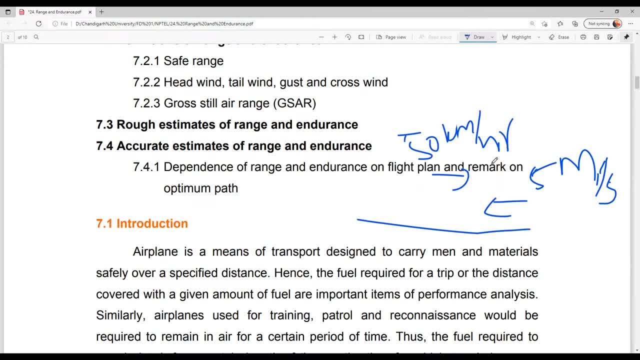 It is normal. So we are going with 50 kilometer per hour, Right, And you will be having a minimum acceleration. You will be using minimum acceleration, But when the speed of wind increases 10 meter per second or 20 meter per second, 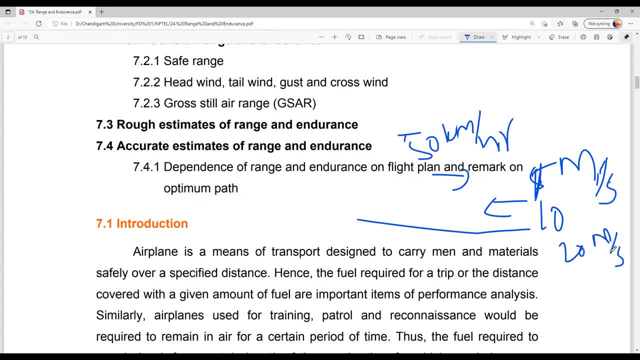 That is huge: Right Turn, 90 percent and 20 meter per second. So what would happen? Your speed will start to decrease. It will come to 30 kilometer per hour With constant acceleration. If acceleration is A is constant. 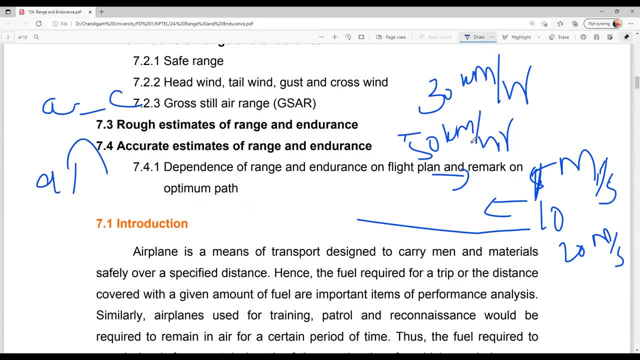 Obviously, you need to increase your acceleration To reach again with 50 kilometer per hour, Right When the wind direction is against you, Right Then it is a vehicle, Whether it is a bike or car or bus, Any vehicle Okay. 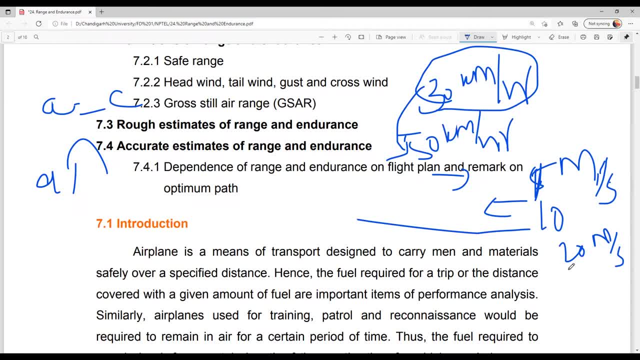 So that same is applicable for aircraft also. So when we are facing a headwind, We will lose the velocity. Okay, So then we have to increase the acceleration. We have to give more thrust When we are flying against the headwind. 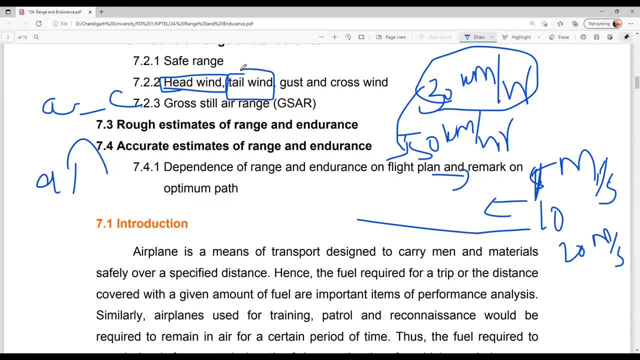 But there is advantage with the tailwind Right, Always there will be advantage with the tailwind So, because it is going to help you to move fast, Faster. So again, let's consider that you are driving a car, And this time you are moving in a speed of 50 kilometer per hour. 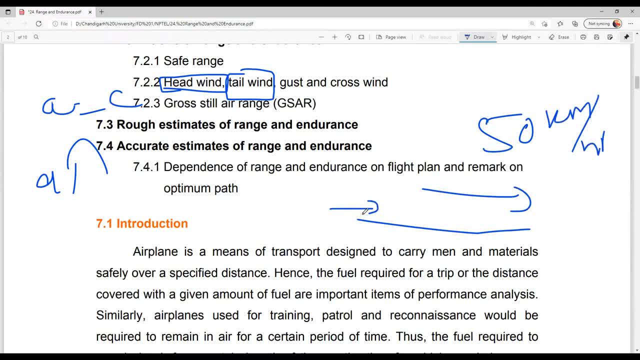 Wind speed is Tailwind winds. it is coming behind you, Okay, Not opposite to you. It is coming behind you, Okay. So 5 meter per second If the wind speed is there, So you will be flying with minimum acceleration. 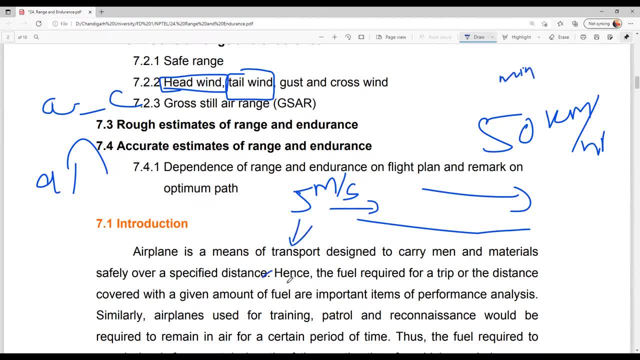 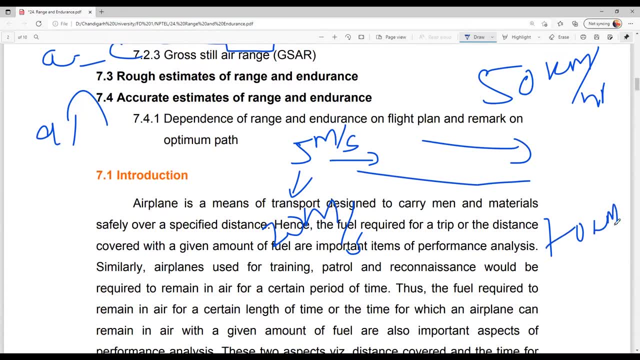 But when speed of this wind increases 20 meter per second, Your speed of the car will be increased 70 kilometer per hour. 70 kilometer. I am just giving the approximate values. Okay, So don't get confused Like this is the exact value. 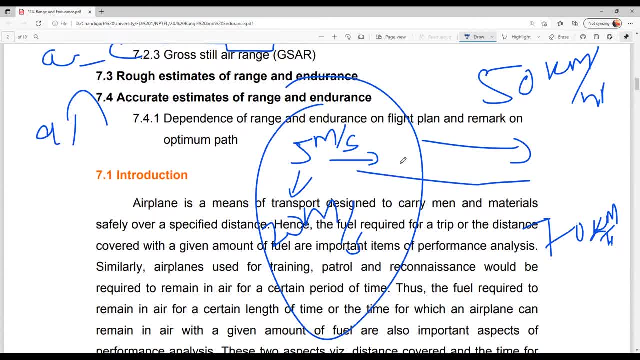 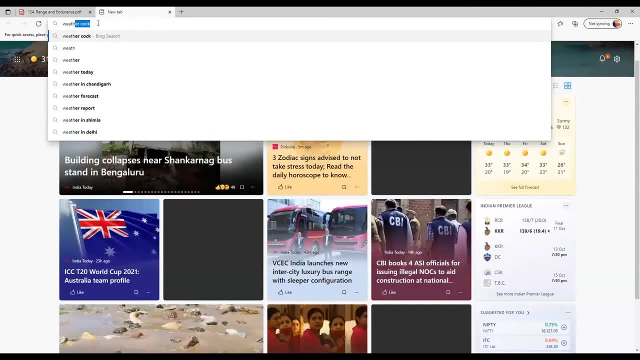 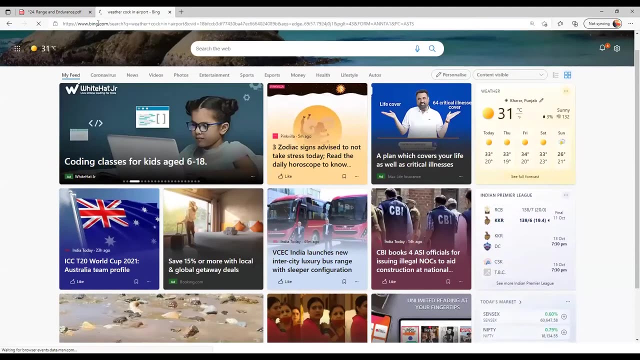 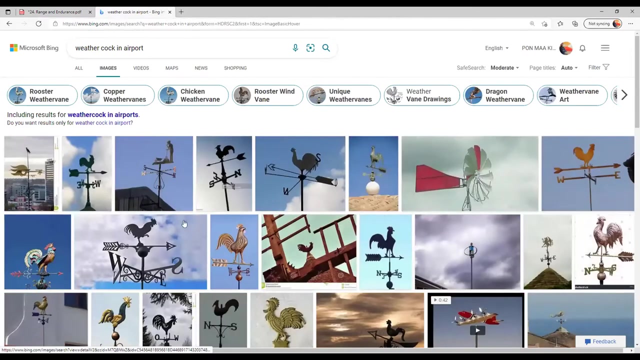 I am just giving an approximate value, So 70 kilometer per hour. These things you can do experimental also. Right, You can identify the wind direction. So wind direction can be identified with weather clock. Yeah, So you can easily identify. 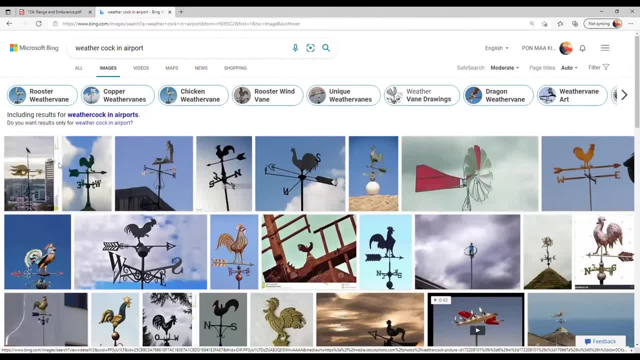 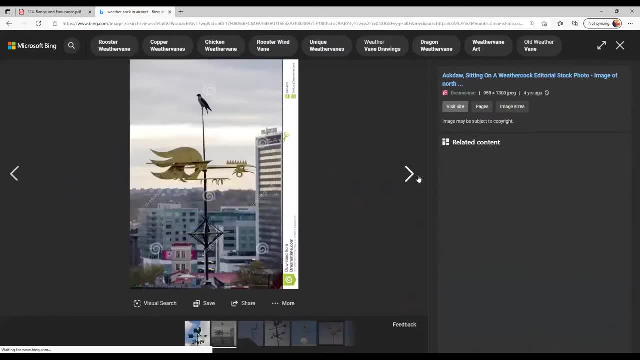 If you are using weather clock system, You can easily identify the Direction of wind. Okay, So this is. This is used for identifying the direction of Weather clock. So in most of the airports They will be having In A wind turbine. 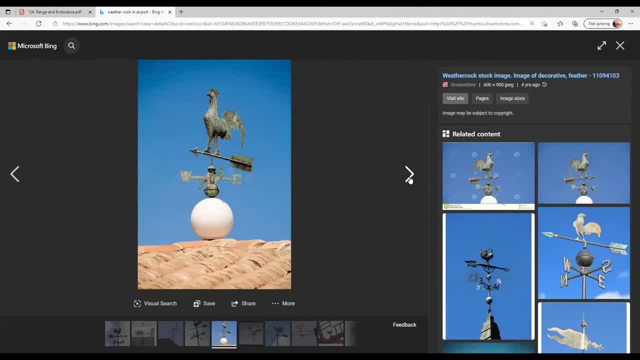 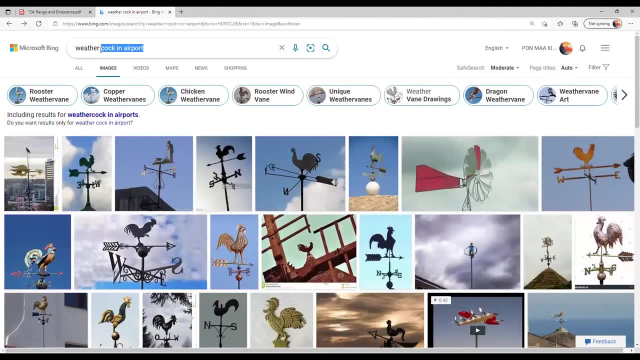 Wind turbine Plates They will be having Right. So this is one of the Good example To identify Which direction Wind is flowing. Okay. So another one is Weather Sock, I think In airport, Okay. 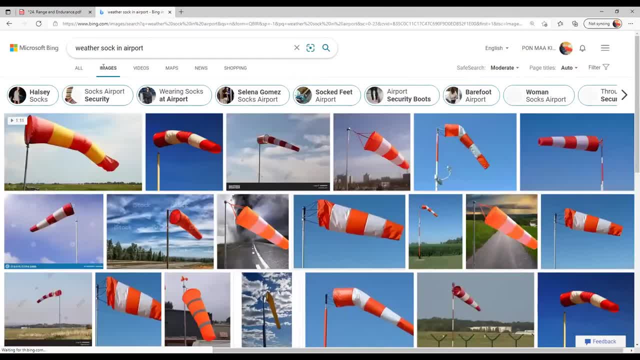 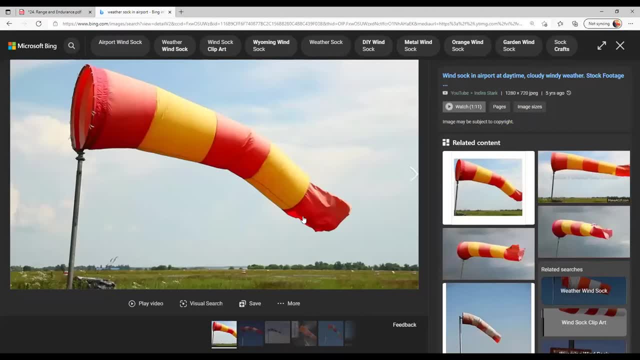 So So Yeah, This is Okay. So this is weather sock, Or wind sock, Sometimes they will call. So this will be used in Every airport Wherever there is a Runway Right. So there are. 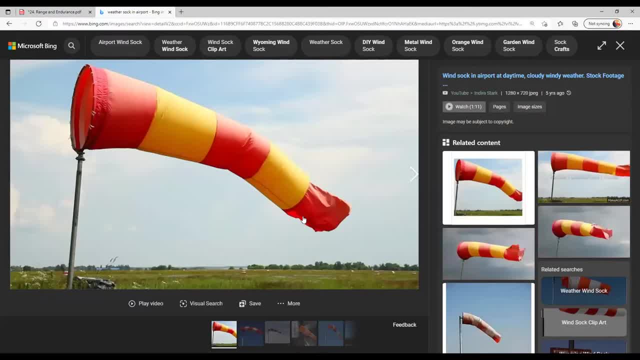 Even private runways Are available in the country, So they will be using This Wind sock. Okay, So they can identify easily Which is the direction The wind is blowing. Okay, So you can drive your car Or bike. 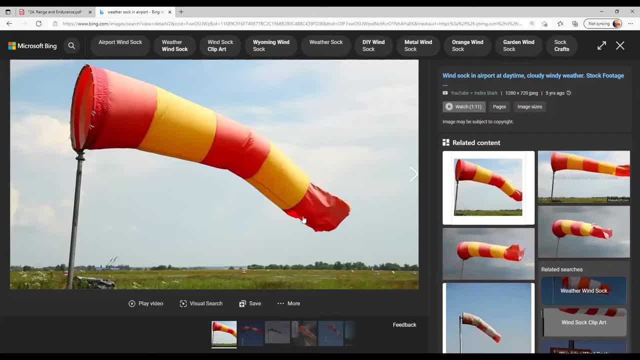 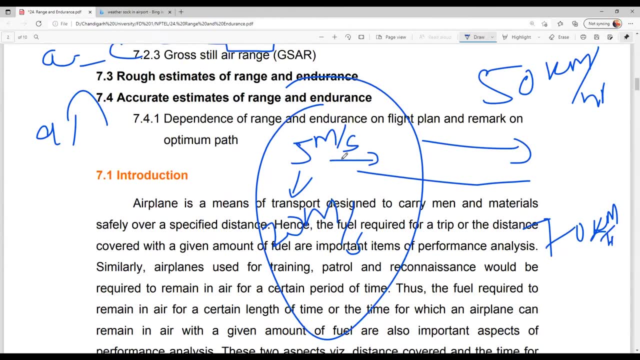 Against the wind And you can identify Which direction The wind is blowing. Okay, And you can Feel the same Thing Like What happens with that. So when we are having a tailwind For our Bike Or car, 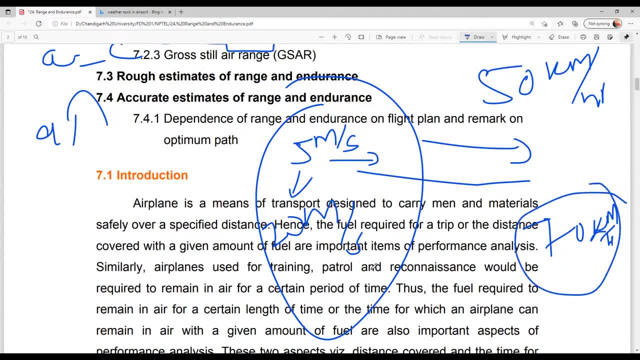 Even for our aircraft, The speed will be automatically Increased Because of the Wind flow. Okay, So it will push you. It will push you forward, Okay, Whereas when there is a headwind, It will pull back, Okay. 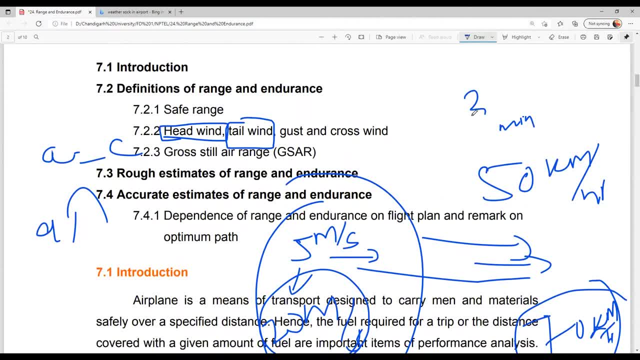 It will pull back, So Speed will be reduced To 30 Km Per hour. Okay, So this is the advantage When we are having Tailwind, So obviously The gustwind And the crosswind For aircraft. 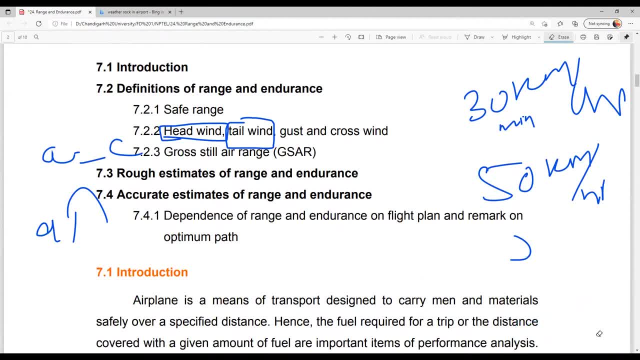 It will deflect The path Right When there is a Crosswind For the aircraft. What will happen? There will be Yaw movement, There will be Sideslip And yaw movement Will be happening. So I am just drawing. 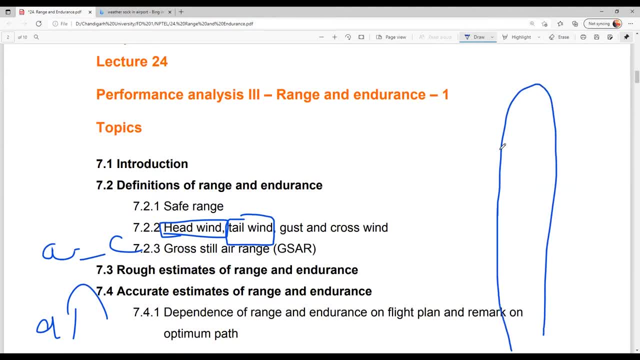 The top view Of the aircraft. So This is the Wind. So If there is a Sudden Crosswind, Okay, So the aircraft Will be Deviated. The aircraft Will be Deviated From its 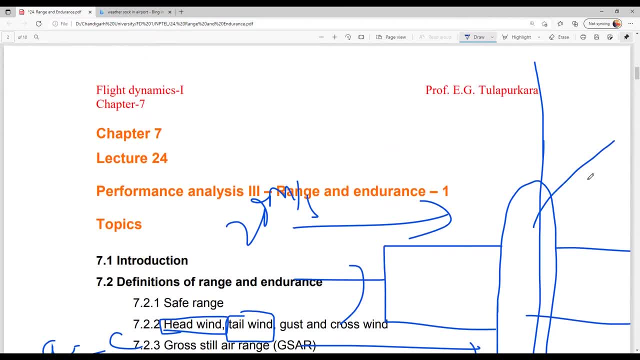 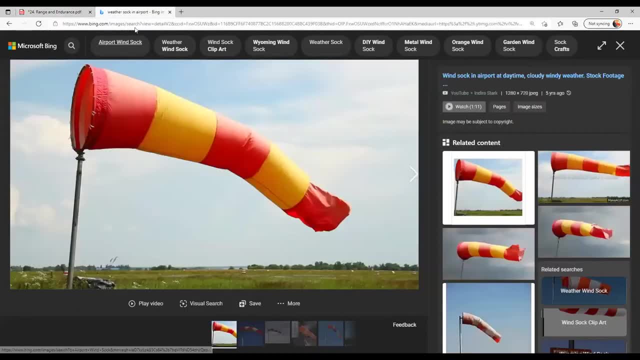 Ojna path. Suppose This is the Ojna path, It will be getting Deviated Because of this Crosswind. Okay, So Crosswind Landing Is Very Worst Thing In the 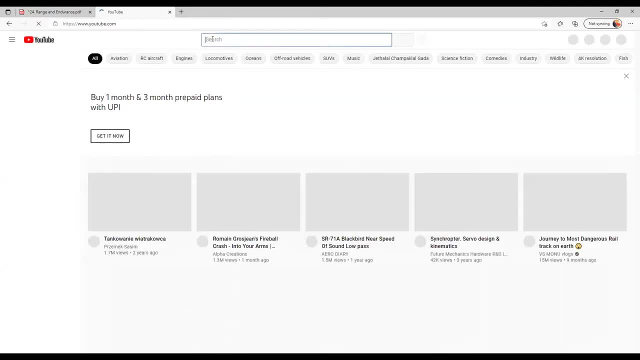 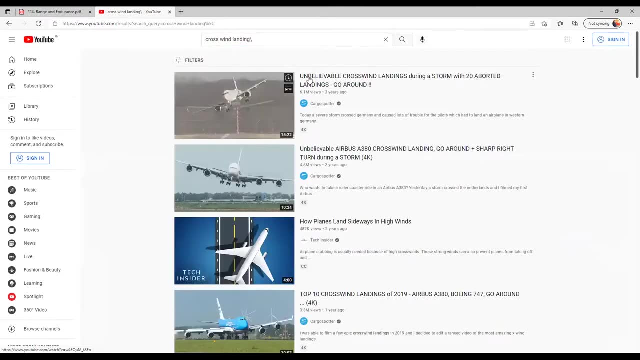 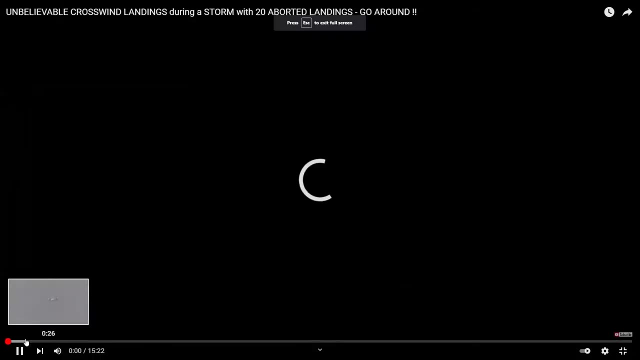 Windy Regions. Okay, So I will show Like. So Here You can see How The Aircraft Is Beginning. So It Is Trying To Come In Ojna. 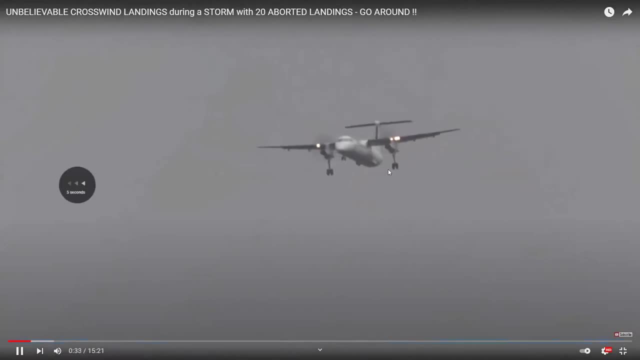 Path But Due To The Crosswind, Obviously The Aircraft Is Having Additionally A moment Right, So This Is Obviously It Is A Dangerous Situation For The 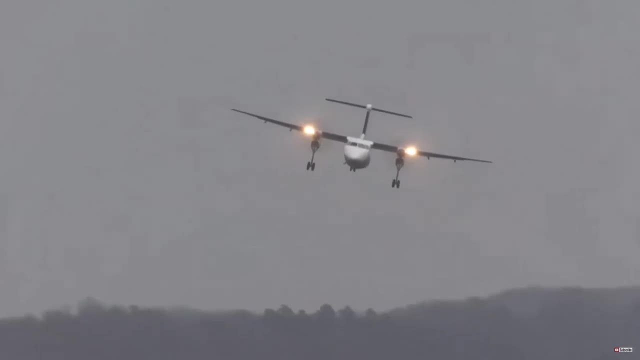 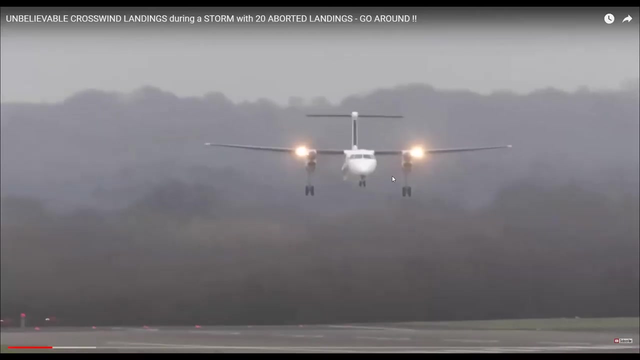 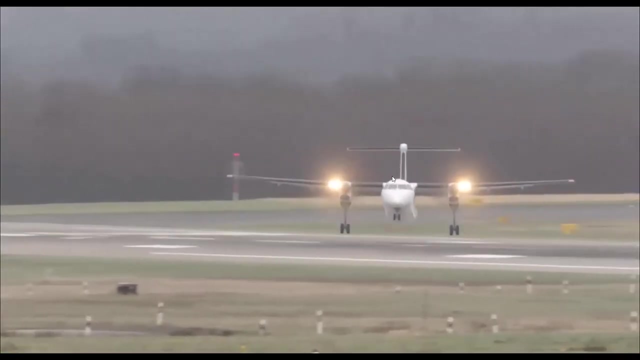 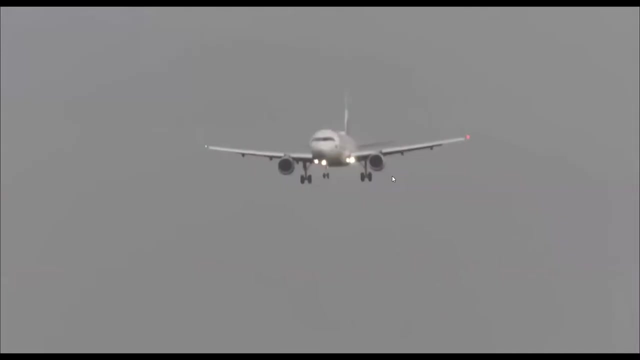 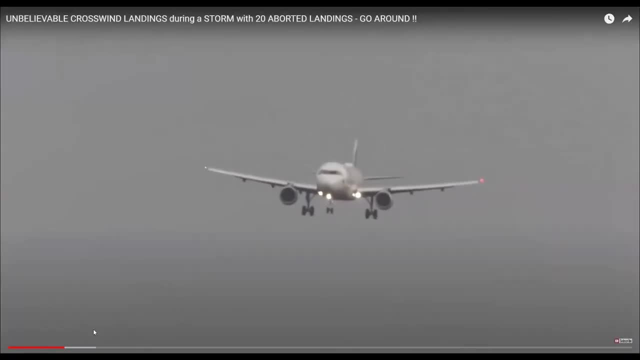 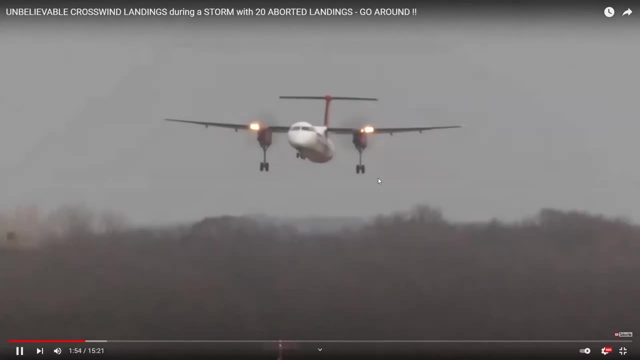 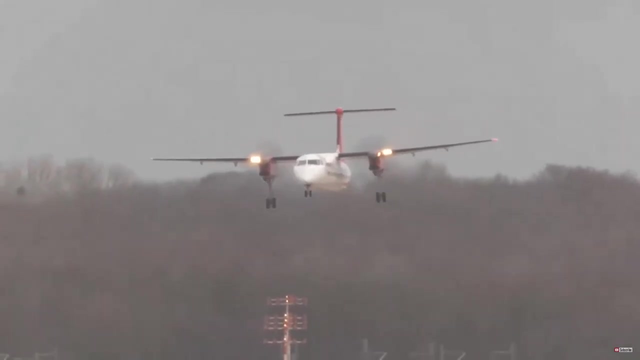 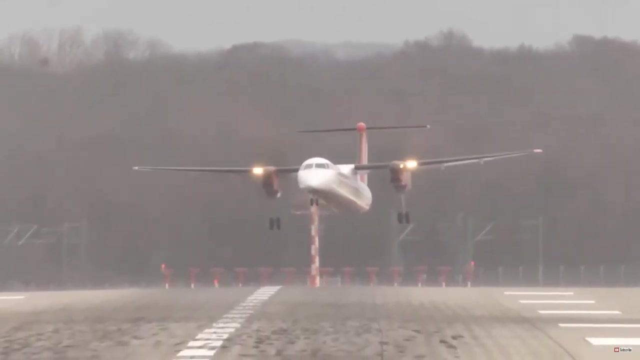 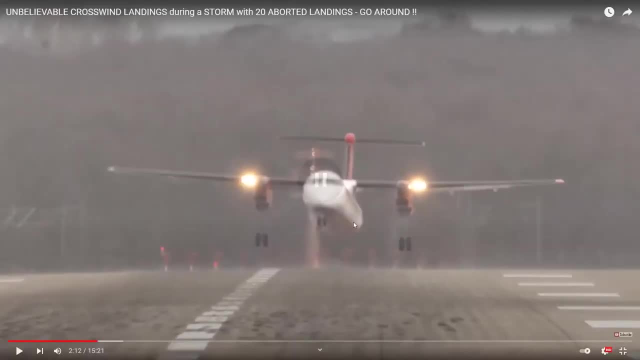 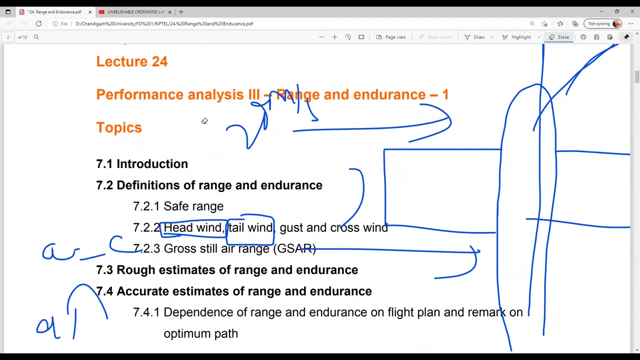 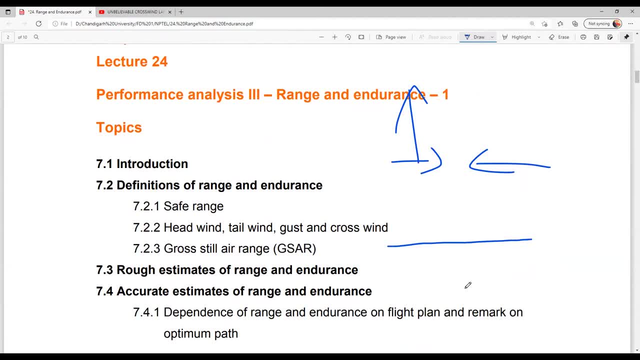 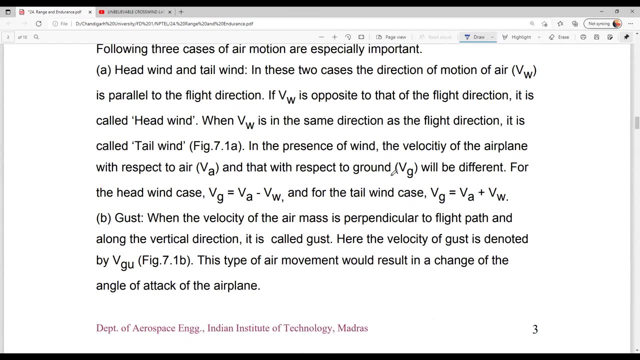 the required altitude is reached in the cruise altitude, so the pilot will prefer tailwind. okay, because we can have good range with less fuel consumption, right, obviously. so that need to be discussed, right. so i hope you got it. what is range and everyone? so this is the parameter they have. 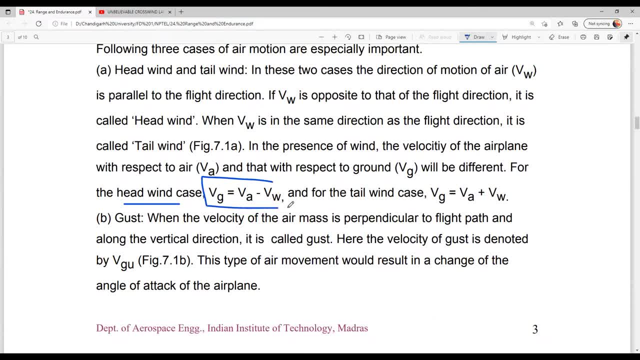 given, like in headwind case, the velocity will be minus right, as i told, from 30 kilometer per hour in headwind. we will be having 30 meter 30 kilometer per hour during headwind. but in case of tailwind we need to add the speed with the velocity of the wind. so if you are flying with 50, 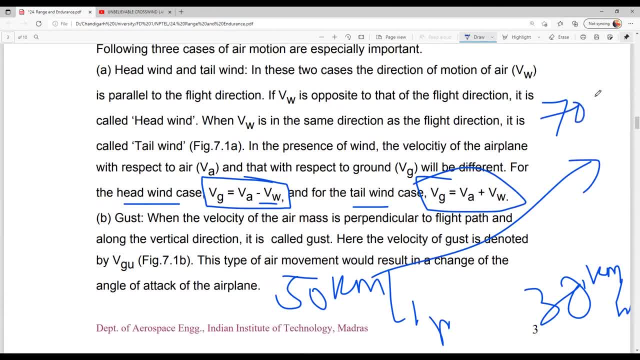 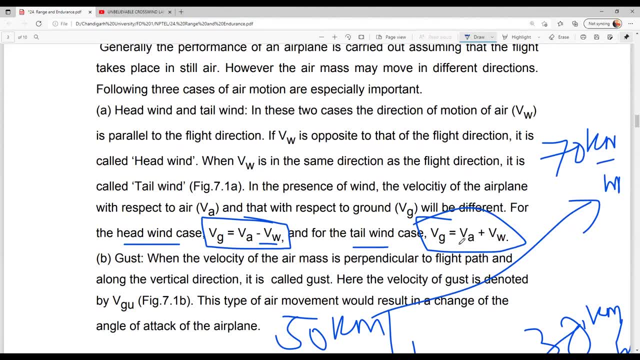 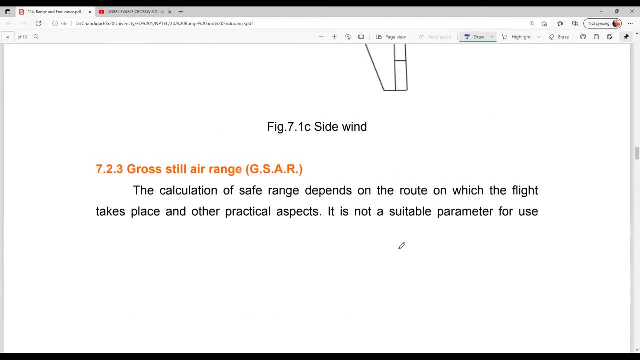 kilometer per hour, then in case of tailwind it is 70 kilometer per hour. okay, just i am giving like a example. so in tailwind you have to add the wind speed, in the headwind you have to subtract the wind speed. yeah, this is. this is the diagram product. so already i have shared this pdf. 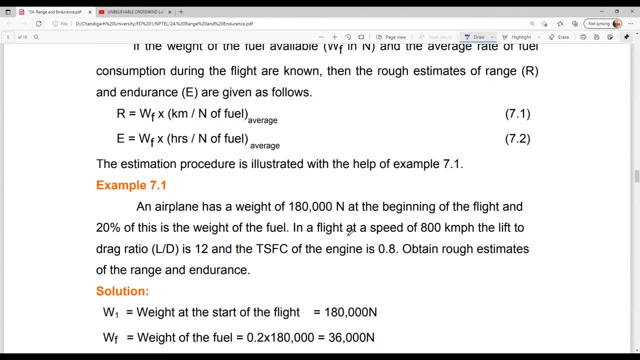 with everyone in this group, as well as in the uh whatsapp group also. i have shared and it is already there in blackboard, so kindly request you to solve. like. whenever you are having time, try to solve the problem. okay, say, previously for flight mechanism, it was five hours, we had tutorial. i. 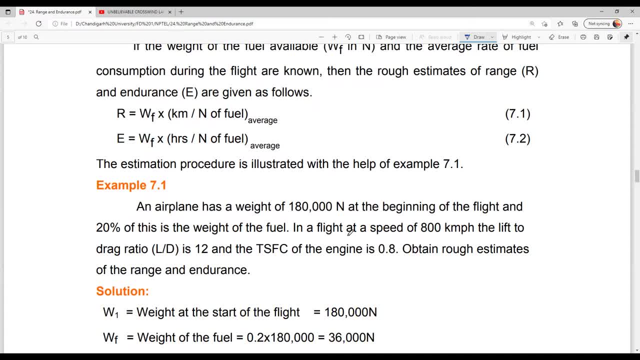 don't know why they have removed the tutorial this time. even i have asked them why you have removed the tutorial, but they said no, no, no, we have to remove that. the tutorial is very much important for flight mechanics. okay, so it is your duty to have that tutorial things solved. 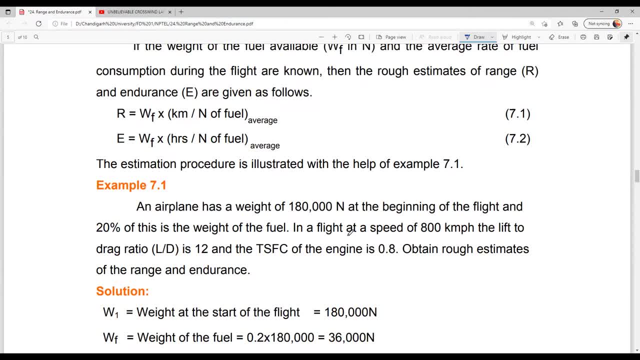 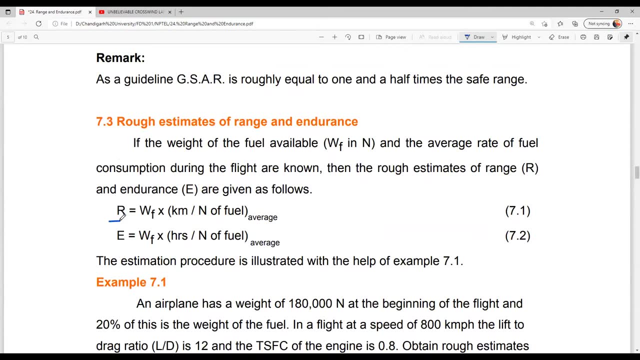 although i am giving that time, but the problem is that you have to do that to your flight mechanics time, but I cannot wait and I cannot ask you to solve That will take much time. So let's see how to calculate the range. So range is given with fuel available. fuel available. 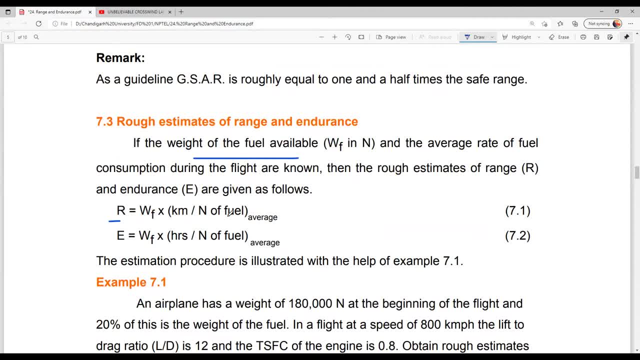 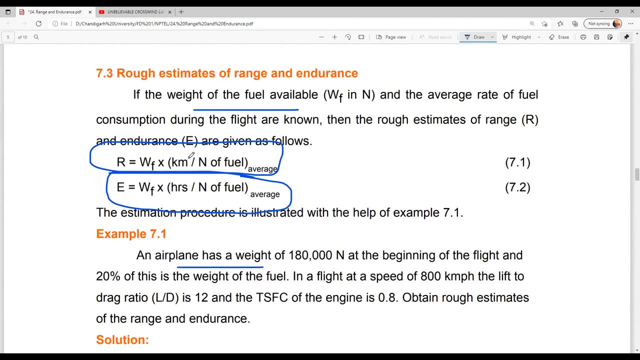 into kilometer per Newton of fuel. So from this, you may feel like how this equation has been described. You may have the doubt, like how the equation has been described. So let's solve this example and then you will understand that. okay, this is the definition. 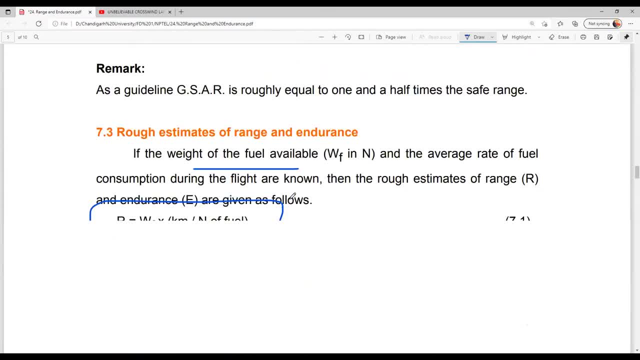 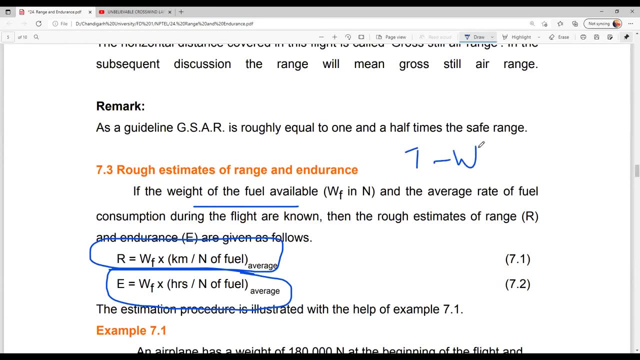 of this equation. So when there is a mathematical equation, there is a definition, also right, Like thrust minus W, of cos. gamma minus drag is equal to 0. So this is for climb, right, This is for climb So. 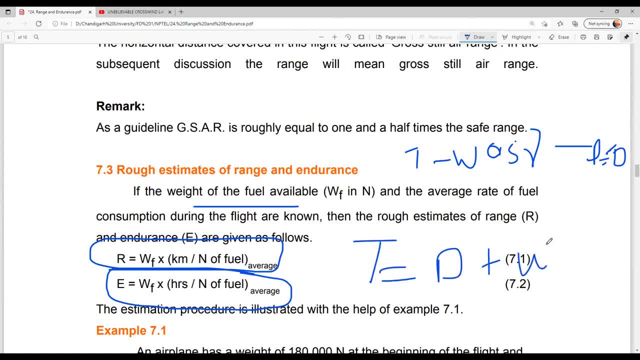 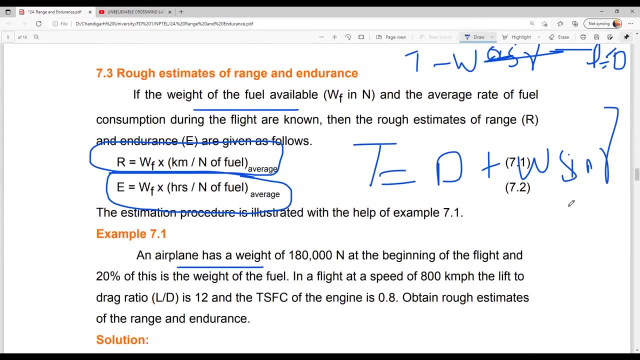 how we are writing. thrust is equal to drag plus W of sin gamma. So this is for climb we have written. So what this equation is actually indicating What this equation actually indicating That you need to know right, Then only you can understand, like how it. 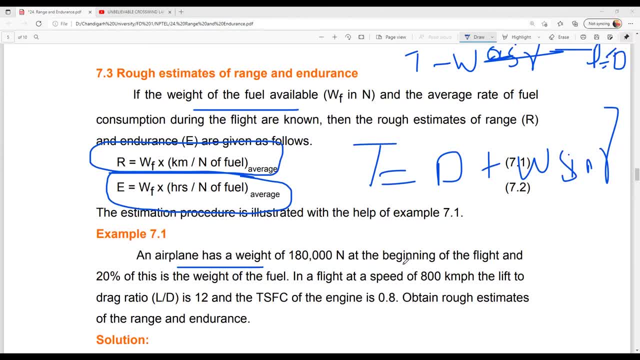 can be how it can be done, right. So let me explain with video, like let me switch on my video and then I will explain. So remember this equation: thrust is equal to drag plus W sin. gamma Thrust is equal. 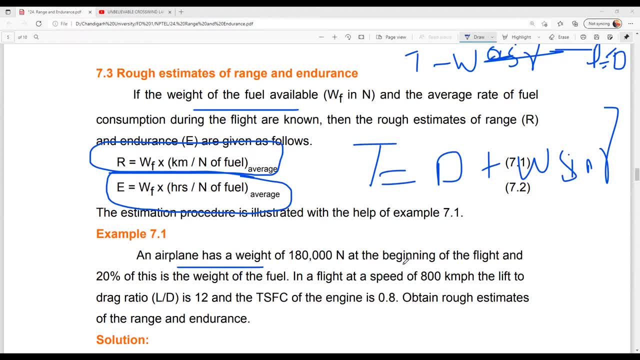 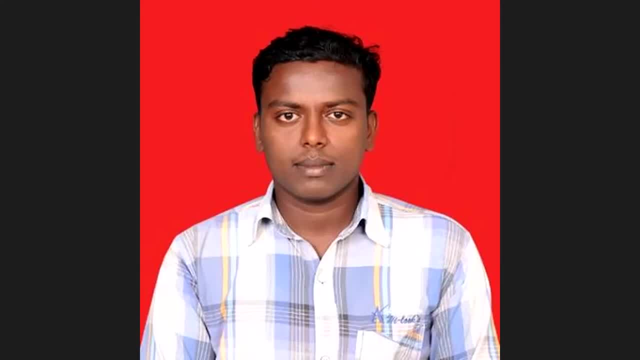 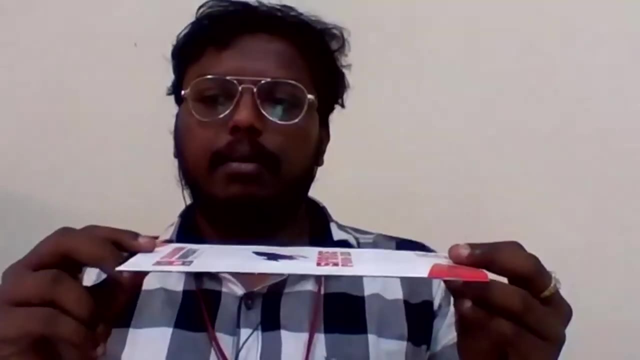 to drag plus W sin gamma. okay, Okay, fine, So consider this is W sin gamma, So let's assume that this is W sin gamma. So let's the aircraft. okay, so we are going to climb. so the equation is: thrust is equal to drag. 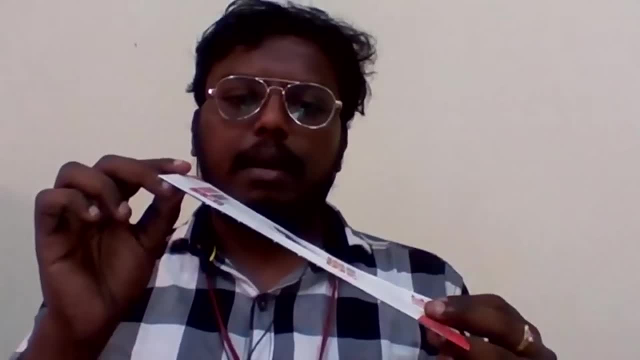 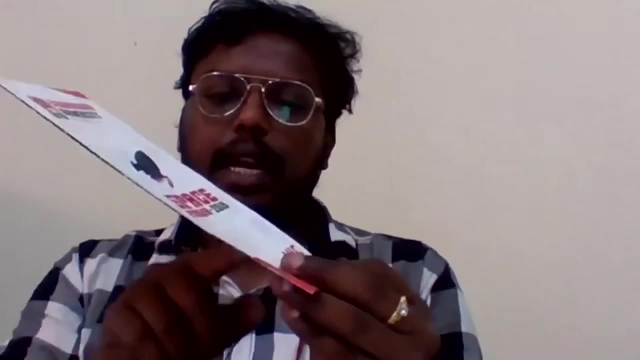 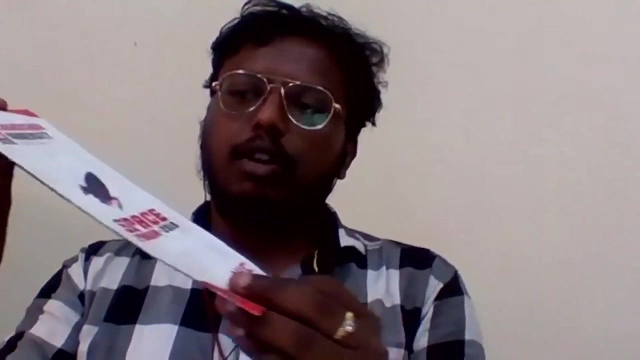 w sine gamma. so when we are climbing winds, we are having an inclined angle right and we are going to climb like this right. we are going to climb like this with the angle of climb. so thrust is a forward force which is going, which is from the engine right obviously. so we are going to move. 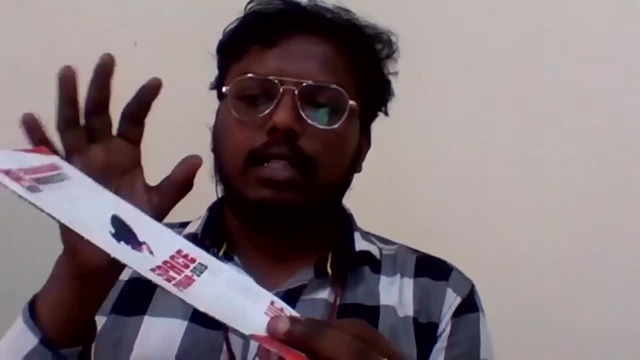 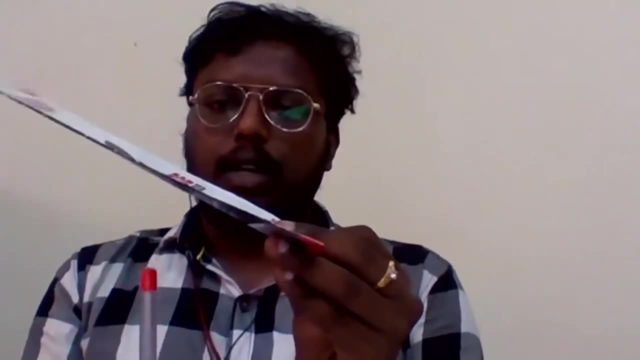 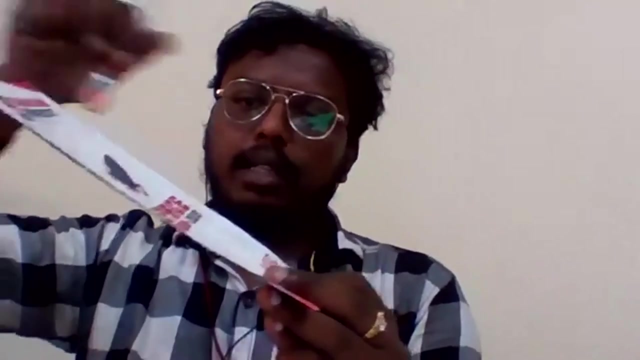 forward. but what that equation depends, thrust is equal to drag plus w sine gamma. weight is acting here right, weight is acting perpendicularly right, but thrust is acting in this direction and lift is acting in this direction, perpendicular to the flight path. lift is acting okay. so when iot is, 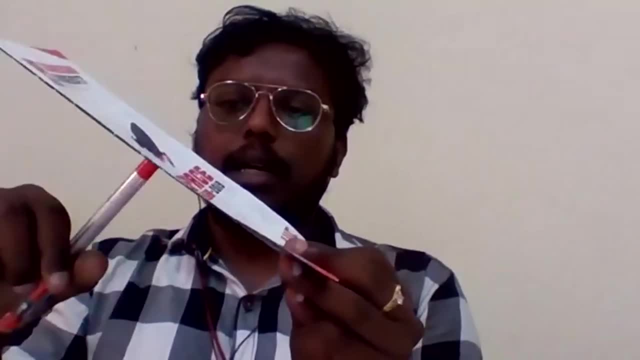 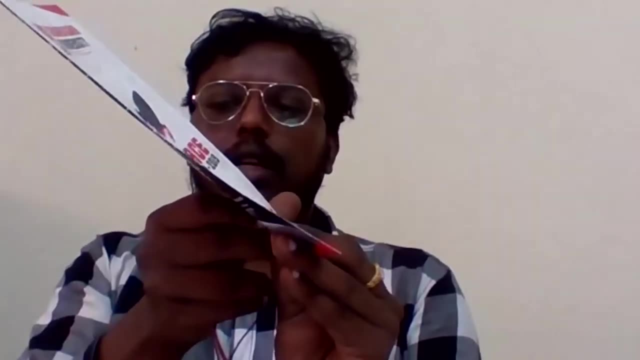 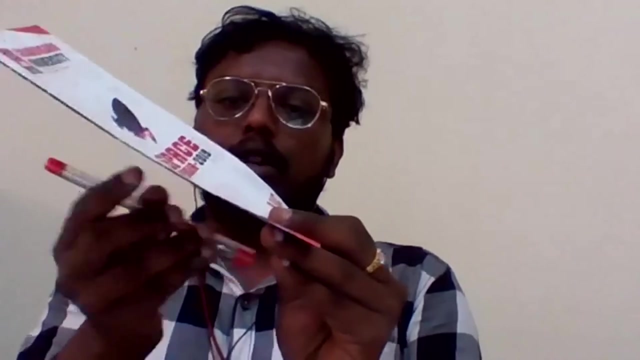 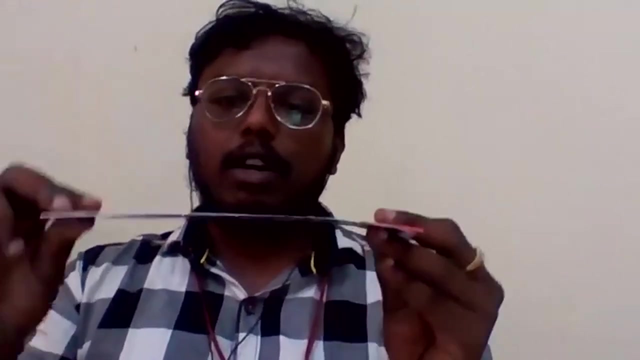 acting. we are making a two components. one is w sine gamma, which is very opposite to lift, lift force w sine gamma. another one is w, sorry, w cos gamma and w sine gamma. okay, w cos gamma and w sine gamma. okay. so w sine gamma is acting along with the drag, along with the drag. so if i want to fly this aircraft in the climb, 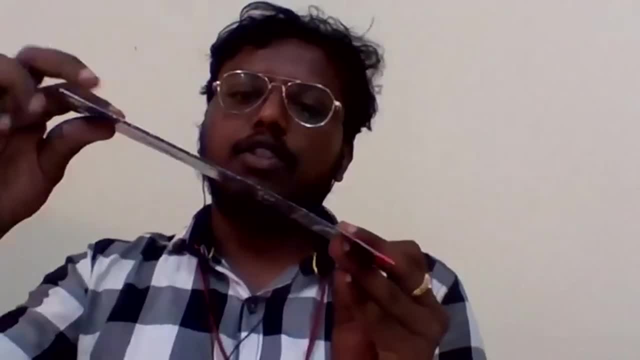 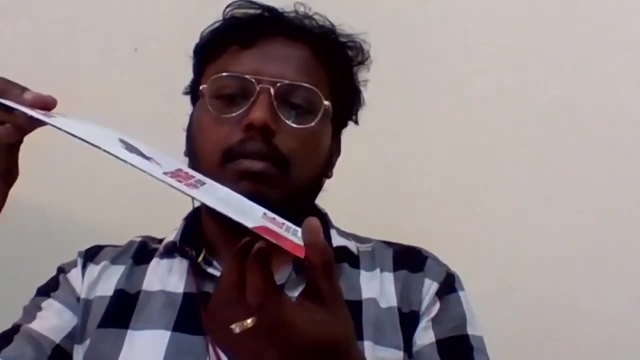 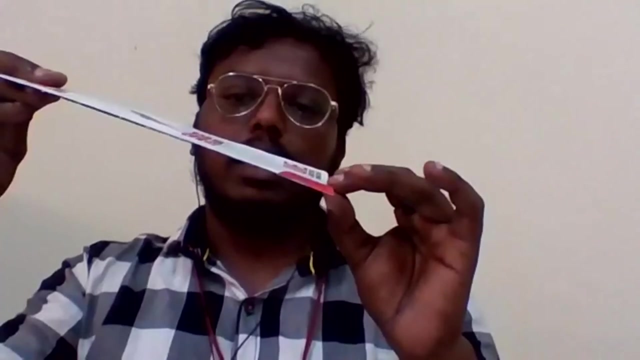 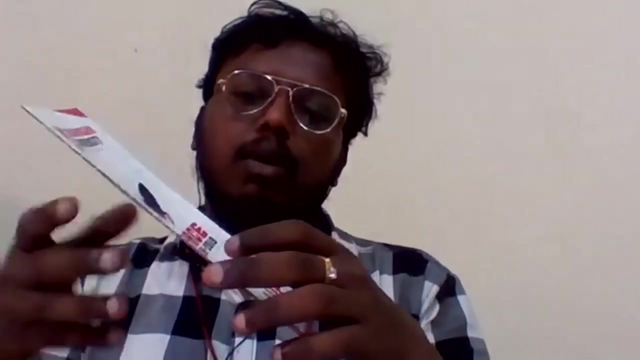 position, i need to generate thrust which will be equal to drag of the structure and weight of the component, weight component. why we? i am saying weight component? because w sine sine gamma is included in the drag force along with the drag force. so we are not only overcoming the drag force, we have to overcome the weight also. so the thrust required at the climb is: 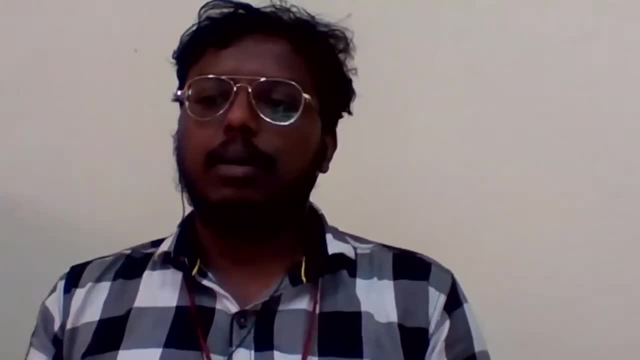 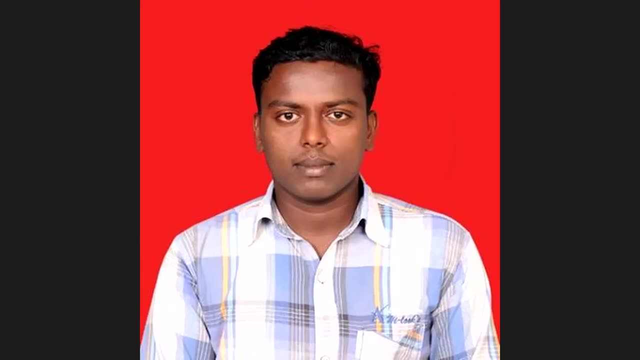 more than the other faces, okay. so that's why thrust is equal to drag plus w sine down, okay. so i hope you can understand that. so, similarly, each and every equation in in this flight market- is not Not only in this, but in any subject you can take- that is, having a definition. 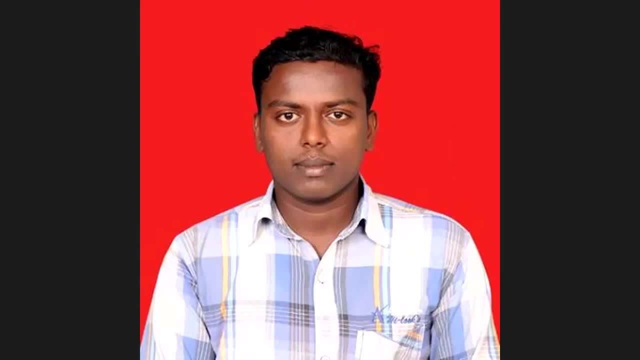 So you should not learn just like that. So if you understand the concept of that equation, then easily you can remember the fact right. So when we are climbing, obviously thrust need to be more. So what are the forces are acting? 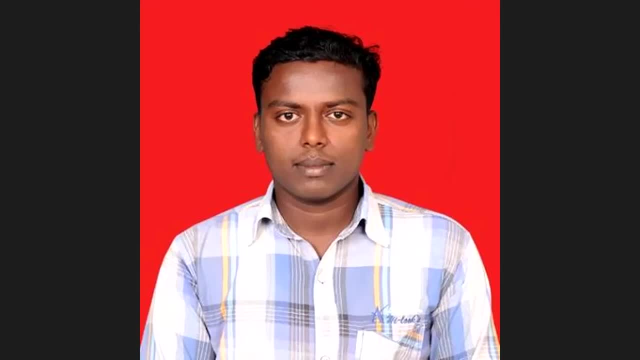 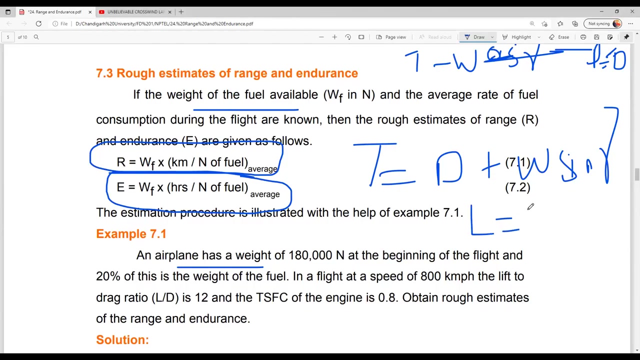 Drag is acting and another component is weight. So weight is W sine gamma, because we are having two components of weight. One component is carried by lift right. One component In the equation- I hope you remember Another equation was W L is equal to W cos gamma. 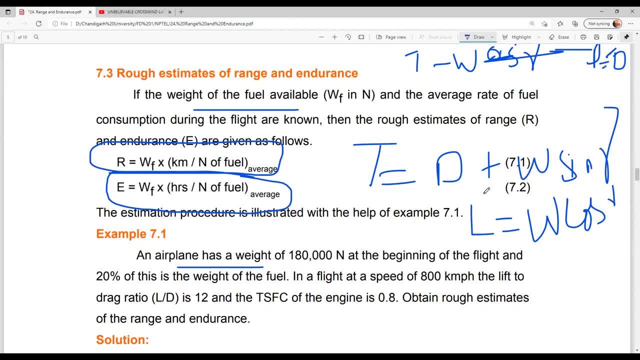 So overall weight is split by two forces. One is lift, is taking care of W cos gamma. Another weight component is carried by thrust. So that is what this equation defines. okay, Right, So you try to learn with that definition. 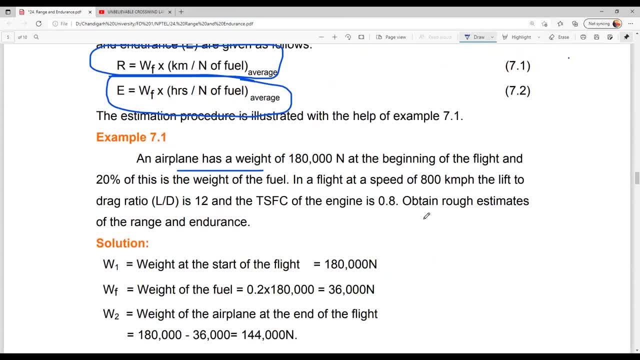 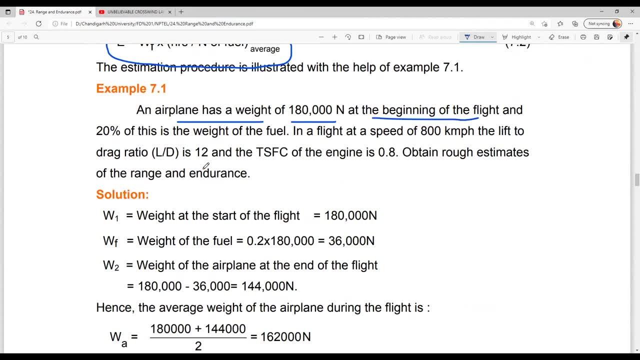 Like how The equations are formed right. So an airplane has a weight of 1,80,000 Newton- 1,80,000 Newton at the beginning of the flight, and 20% of this is the weight of the fuel. 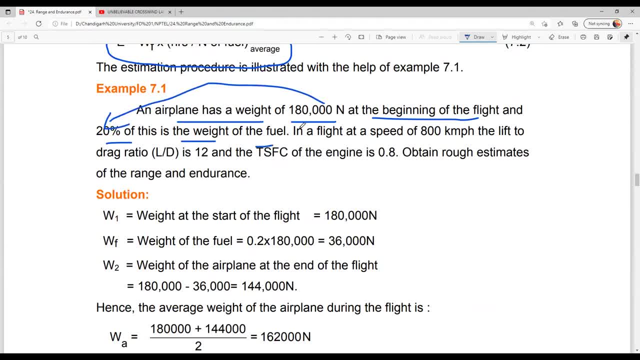 So from this you have to take 20%, that is the weight of the fuel. So in a flight at a speed of 800 kilometer per hour, So aircraft speed is given, The lift to the drag ratio is given. 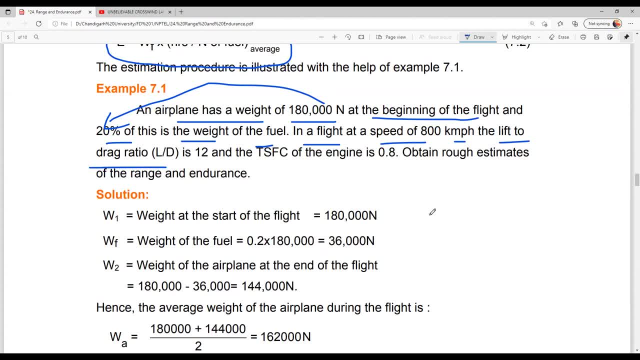 L by D ratio is given Lift to drag ratio. So L by D is also called as aerodynamic efficiency, Aerodynamic efficiency, So remember that, okay. Aerodynamic efficiency And thrust: specific fuel consumption of the engine is given. 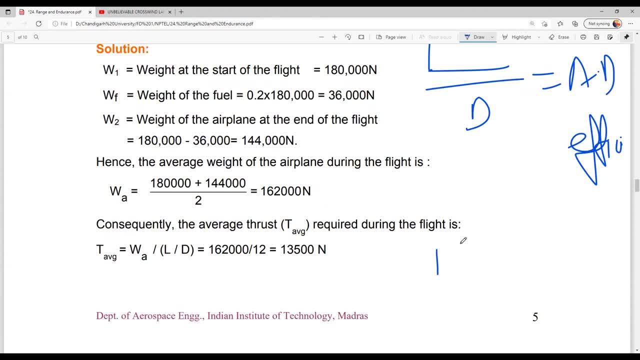 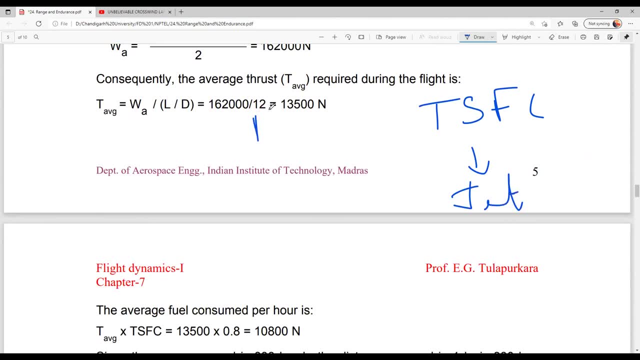 Thrust specific fuel consumption. So when they use the word thrust specific fuel consumption then we can consider this as a jetter. When they are using BSFC, Then we need to go for turbo pro or propeller piston engine combination. propeller piston engine combination- okay. propeller piston engine combination: okay, BSFC. 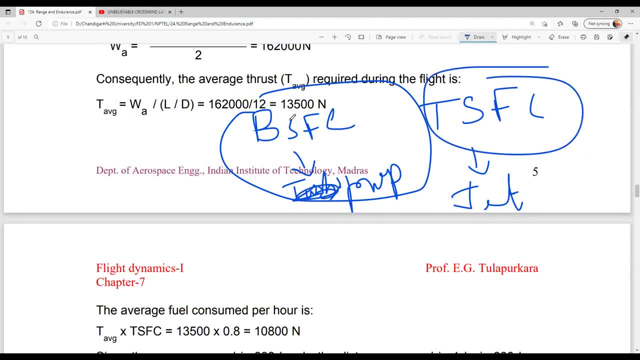 So BSFC is related with thrust. This is given with piston propeller engine. BSFC is given with piston propeller engine. okay, brake specific fuel consumption: This is thrust specific fuel consumption. So that is the difference, Right. 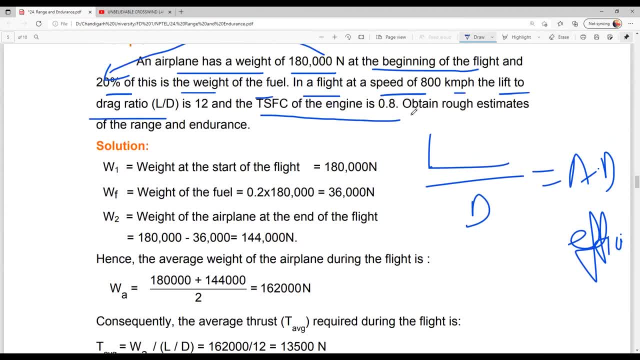 So what we need to obtain is obtain rough estimate of range and endurance. So we have to calculate how much range and how much endurance we have. Okay, So if we calculate that range and endurance, that is fine, Right. 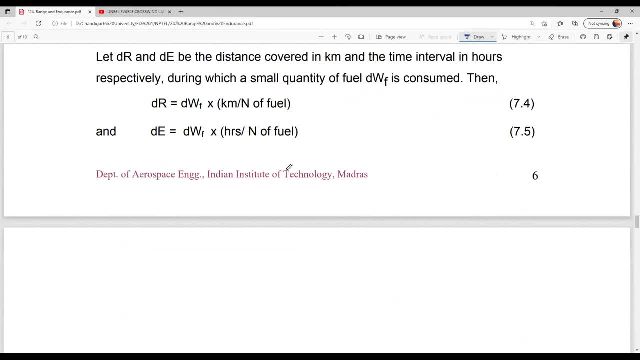 So I will solve this problem, along with another problem we are having, like in the next class, which is very similar to the range and endurance.